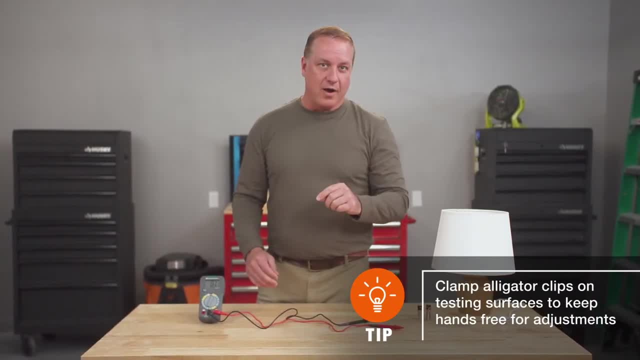 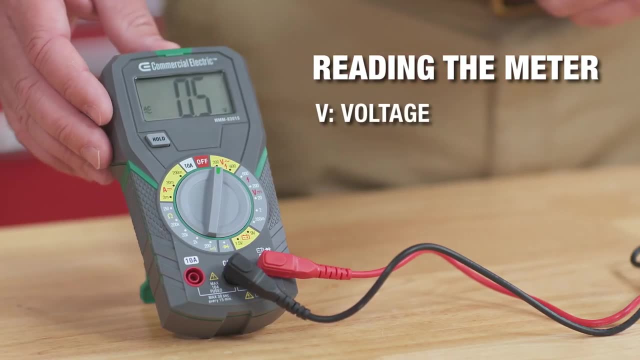 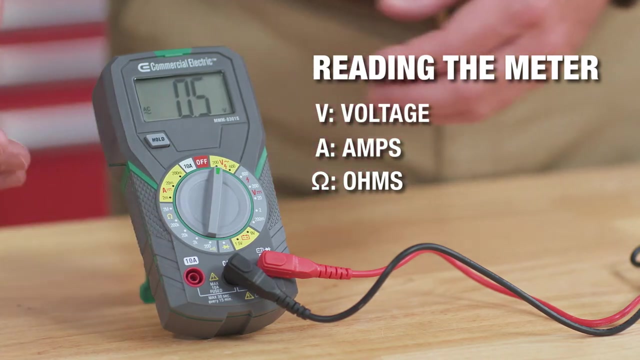 or frequency. It's the positive or hotness. The red probe plugs into the port for the unit or property or hot wire To read the meter. it helps to understand the symbols. V stands for voltage, A stands for amperes or amps. This is the symbol for ohms, M is milliamps, which are tiny fractions. 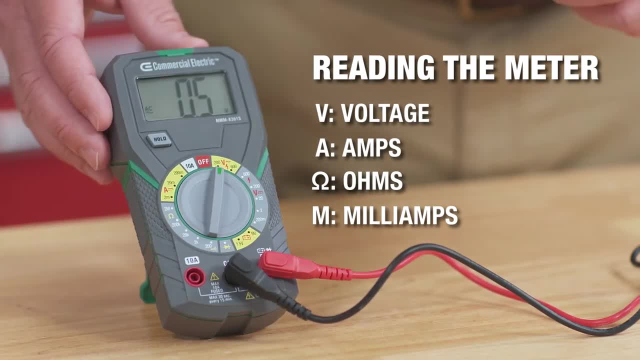 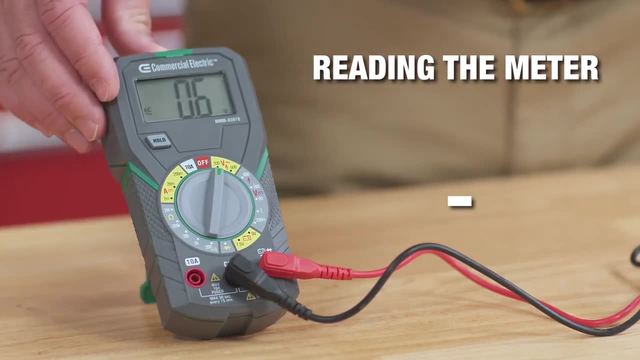 of amperes. Each one is one one-thousandth of an amp. A wavy line indicates an alternating current. A straight line indicates direct current. The red probe plugs into the port for the unit or property or property. The blue line indicates direct current. Before you begin, check for cracks on the 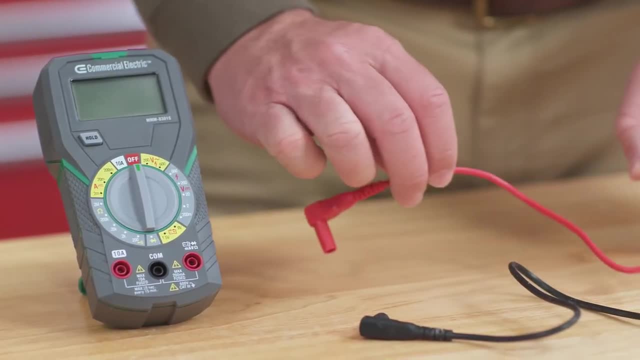 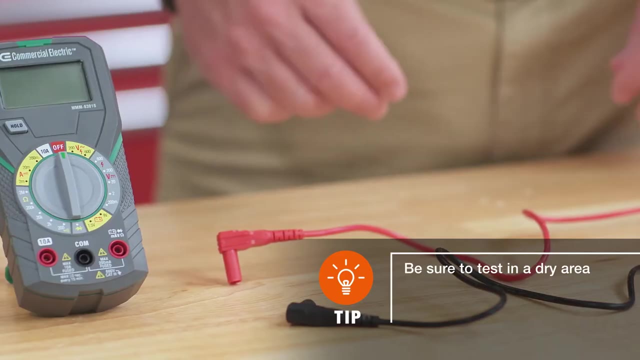 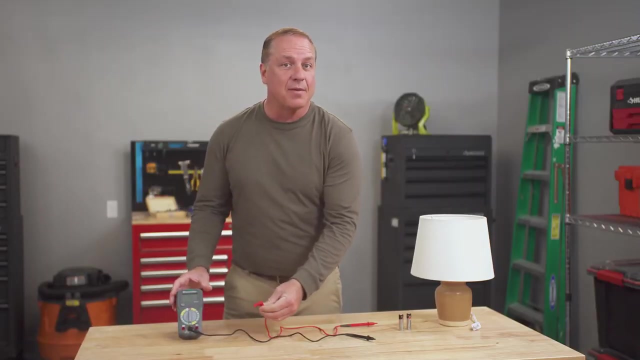 multimeter and for any fraying or nicks on the wires. Next, check that your probes are working internally. This is sometimes called ohming out the leads. Plug the black probe into the common port. Insert the red probe into the jack marked for ohms. Set your multimeter to the ohm meter on. 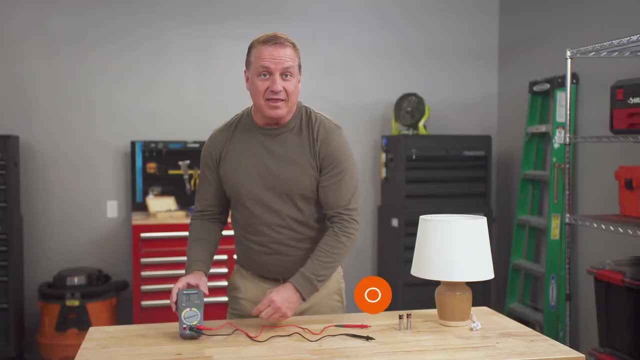 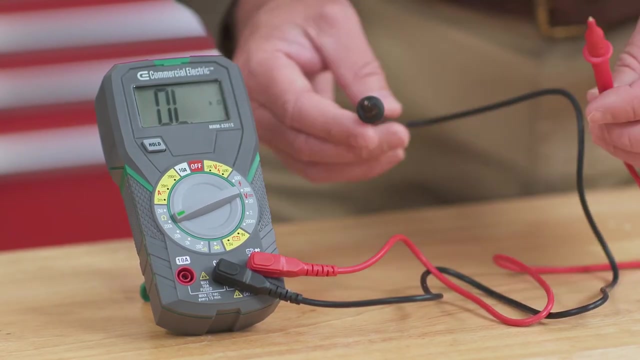 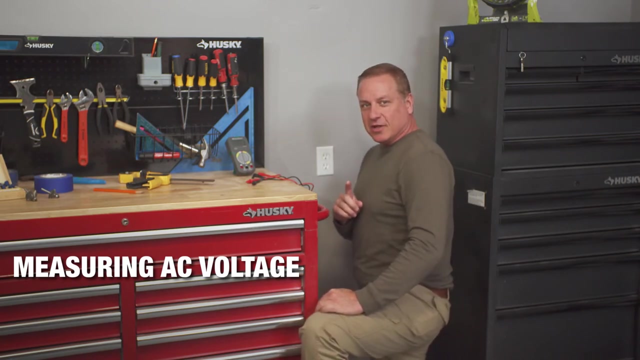 the selector knob, Then gently tap the red and black tips together. Your reading should be 0.5 ohms or less. If your reading is higher than that, replace the probes. Measuring AC voltage is the most common usage of a multimeter. Follow these steps to check an outlet If you're testing another electronic. 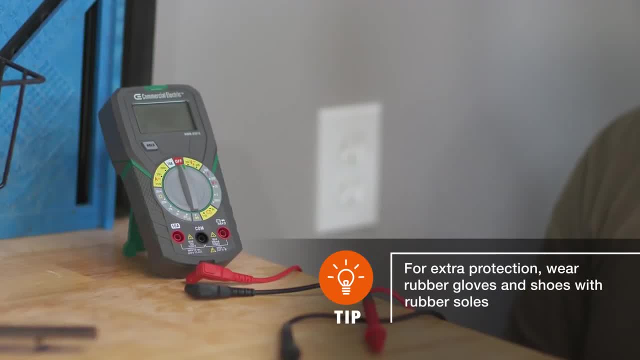 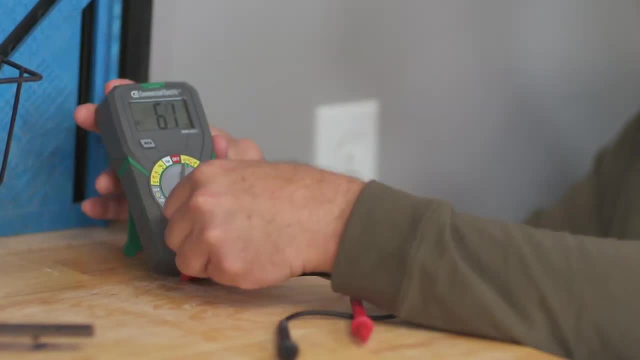 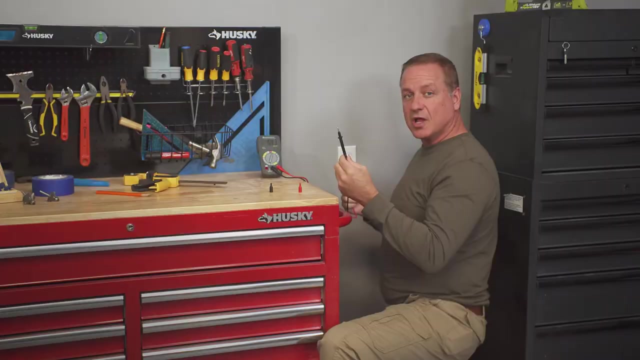 device. the concept is the same. Set the mode on your multimeter to AC voltage. Connect the black probe to the common jack on the multimeter. Plug the red probe into the jack labelled as AC voltage. Place the end of the black probe into the neutral slot On a polarized plug is the wider 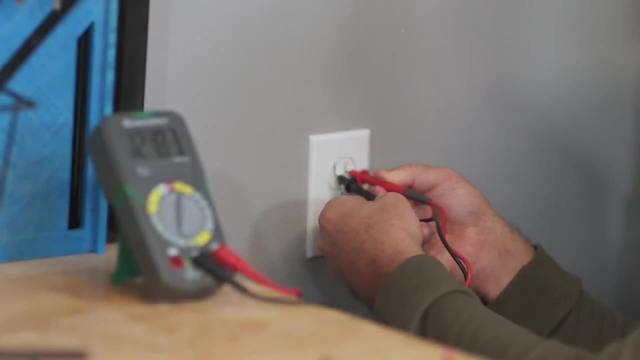 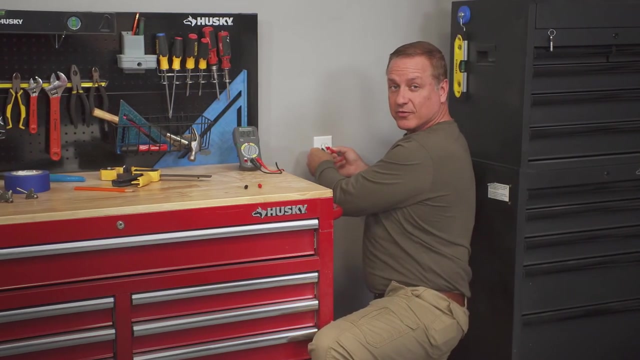 prong. Put the red probe into the hot slot on the plug, the smaller slot. Check your reading. it should read around 120 volts. When you're done, remove the red probe, then the black, from the item you're testing. 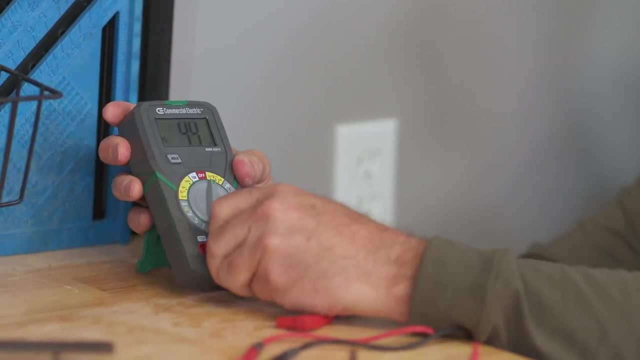 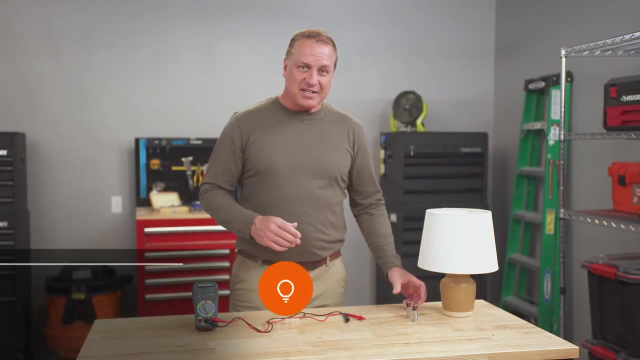 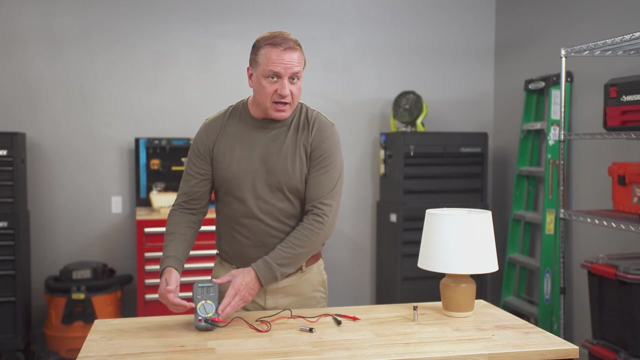 the probes from the multimeter in that same order. you can also use the multimeter to check DC voltage in a battery. disconnect the battery from any power tools or chargers. set your multimeter to measure DC voltage. use the selector knob or button to choose the expected measurement, for example a double.